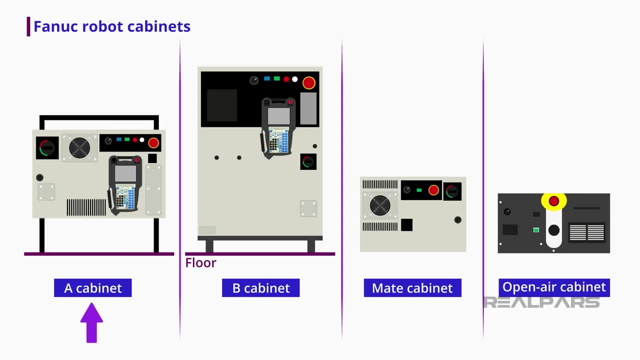 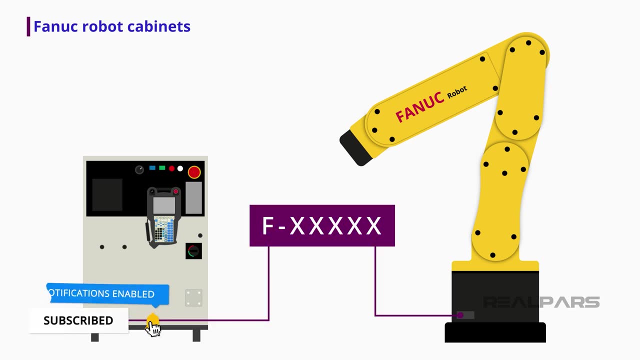 The A Cabinet usually sits on a stand or some sort of structure off of the ground. The Make Cabinet is smaller than the A Cabinet. The Open Air Cabinet is easily identified by the black color. Each robot will have a designated F number somewhere on the controller. 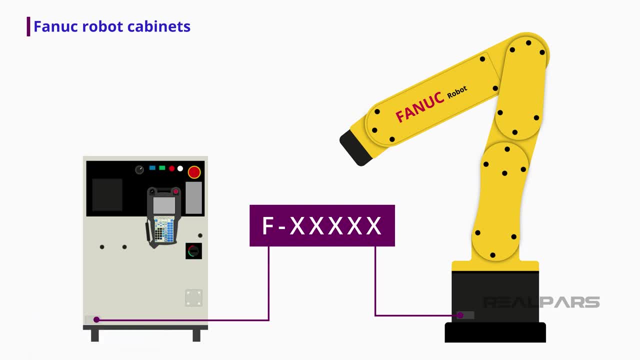 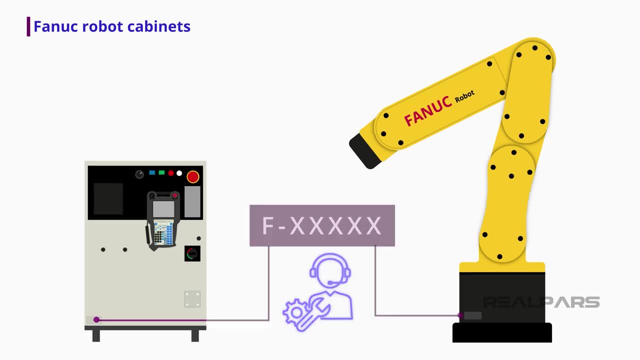 The F number is the serial number for the robot's mechanical unit and the controller. The F number is critical when calling Phanic for technical support or spare parts. As a side note, each robot will come from Phanic with a CD-ROM compact flash. 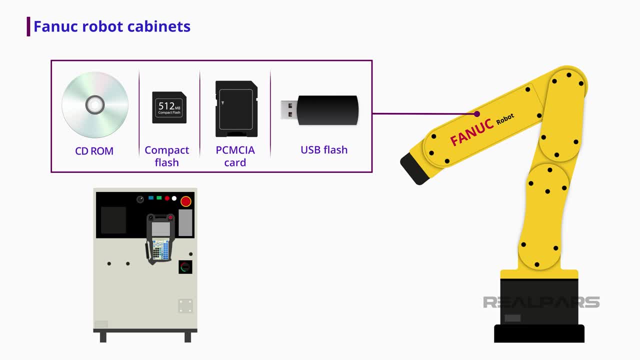 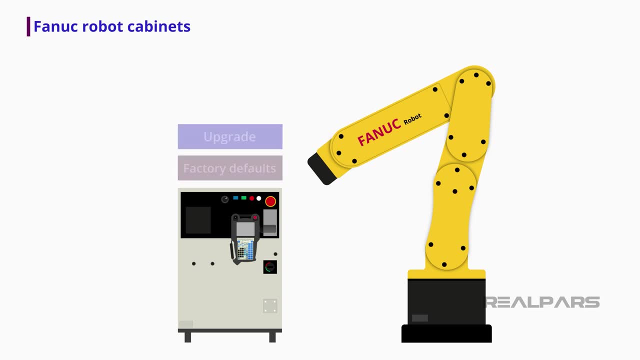 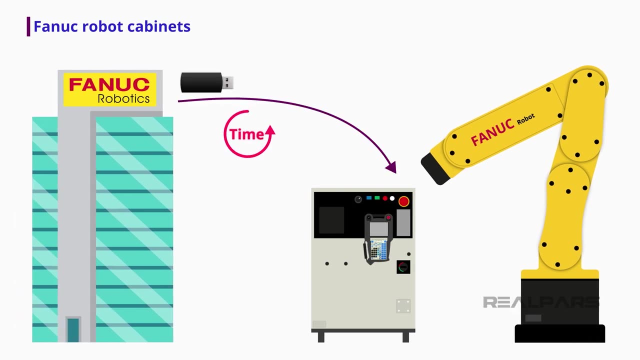 PCMCIA card or USB flash drive which contains software that can be used to revert the robot to factory defaults or to upgrade its features. It's important to know where the media drive is at all times. A copy can be sent from Phanic, but this usually takes time. 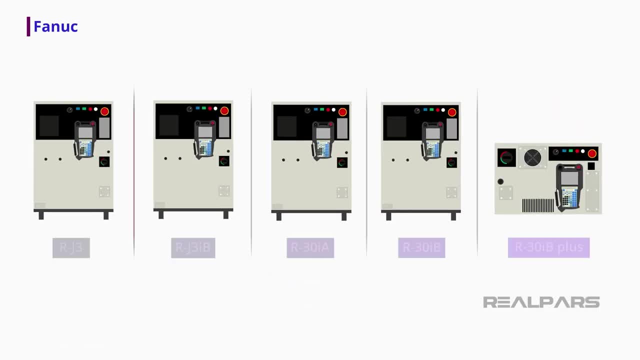 and adds to the cost of shipping the media drive. There are five models of a Phanic robot controller. from oldest to newest, they are RJ3, RJ3iB, R30iA, R30iB and R30iB+. 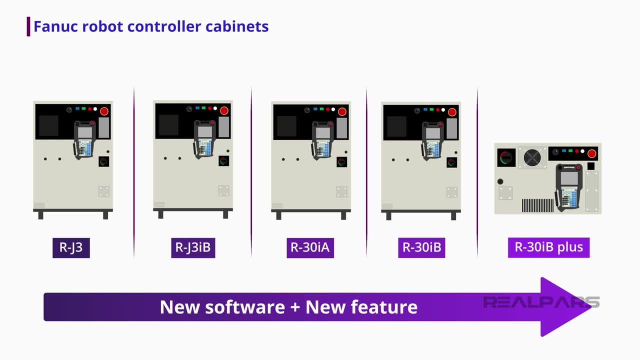 Each controller has a different set of software that has added features on top of the previous version. The important thing you need to know about a Phanic robot controller is that there may be a difference between them, even though the cabinets might look similar. Each controller has its own set of manuals. 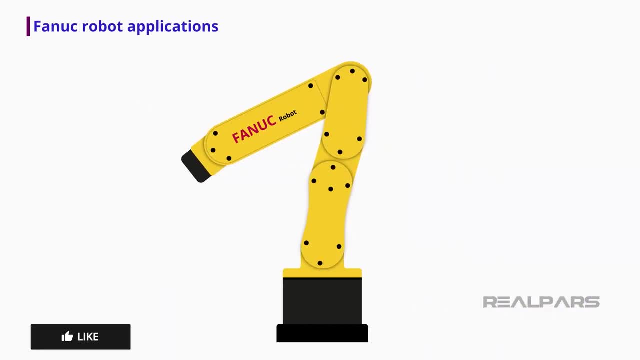 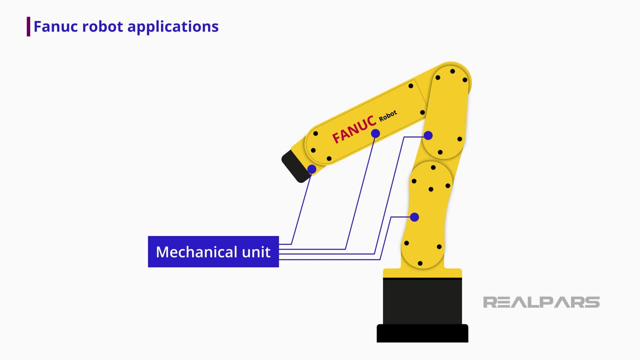 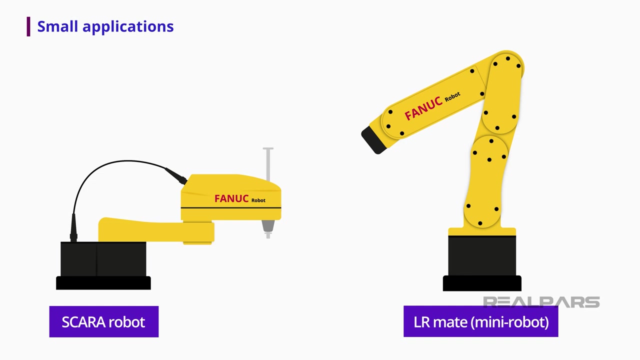 which can be found on Phanic's website. A Phanic robot has a moving structure which is called a mechanical unit. There are many mechanical units and they vary depending on what the robot needs to do. For small, fast and light functions, an LR-Mate mini robot or SCARA robot might be your choice. 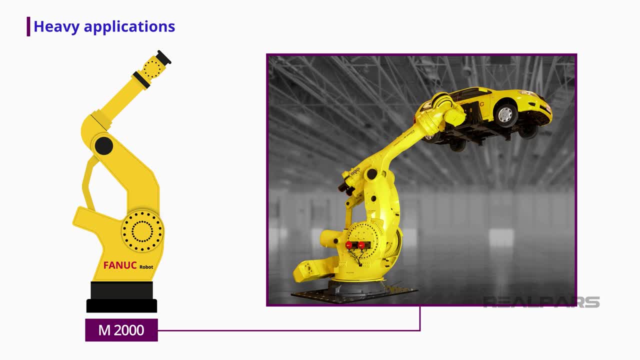 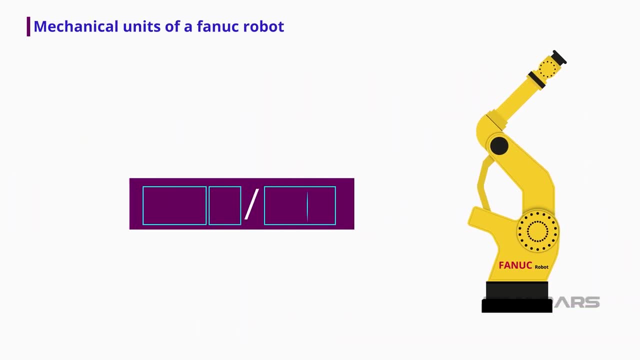 For heavy applications, such as moving things that are as heavy and large as a vehicle, an M2000 will be a better choice. Each unit is designated by a set of numbers and letters. The first number denotes which kind of robot it is. 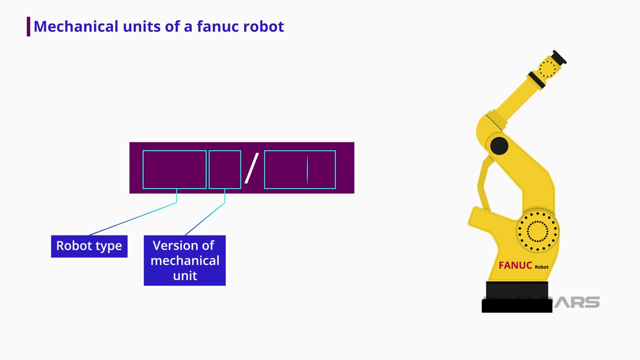 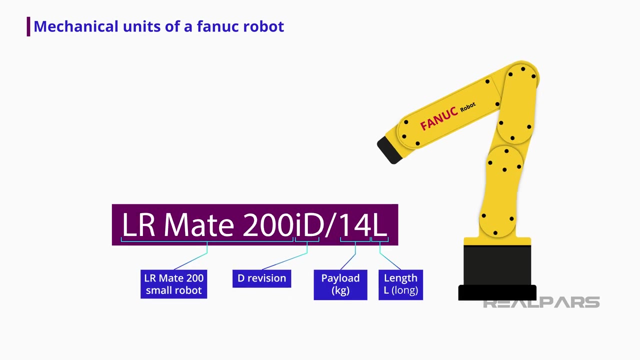 Next is a letter that denotes the version of the mechanical unit. The number after the forward slash will denote the payload of a non-standard robot. The last letter will describe the option of length, usually longer or shorter than the standard. For example, an LR-Mate 200ID-14L is a small robot. 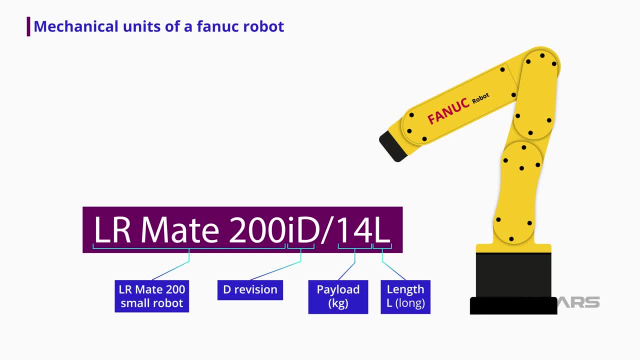 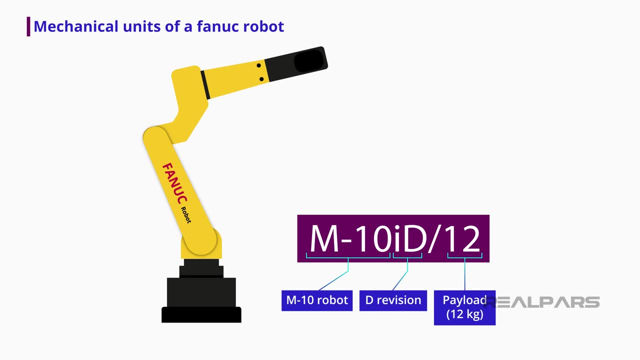 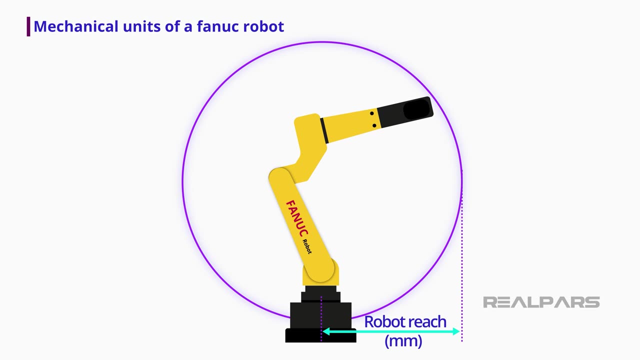 with a D revision that has a 14 kg payload with a long reach. Another example is an M10ID-12, which is an M10 robot with a 12 kg payload. Each robot has a designated reach, which is called out in millimeters. 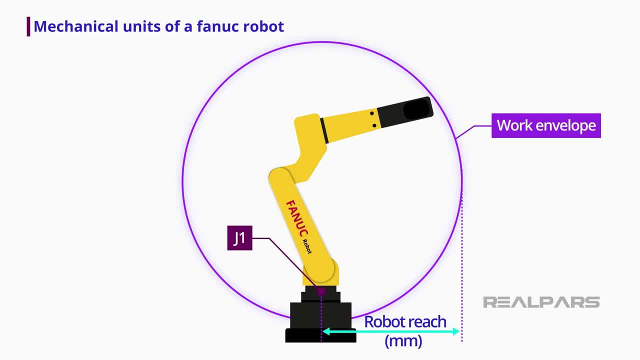 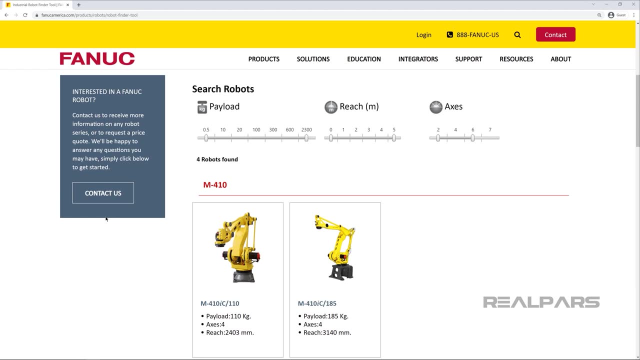 Each robot also has a work envelope to show how far the robot can turn. in reference to J1.. You can use the Robot Finder tool from Phanic's website to help you identify which robot should be used for your application. You can find the link to this page in the video description. 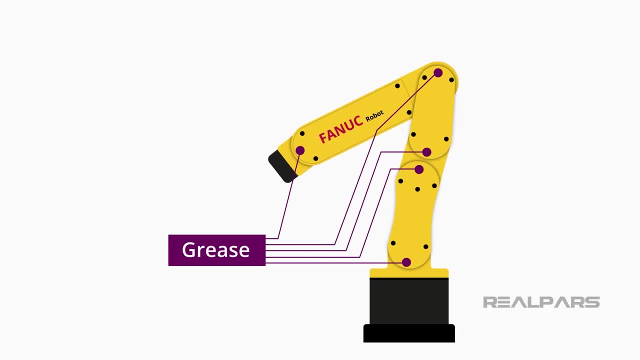 It is also important to remember that each mechanical unit uses grease to lubricate each joint of the robot. Like the oil in your vehicle, the grease needs to be changed periodically. Be sure to check your robot's mechanical unit maintenance manual for more details. 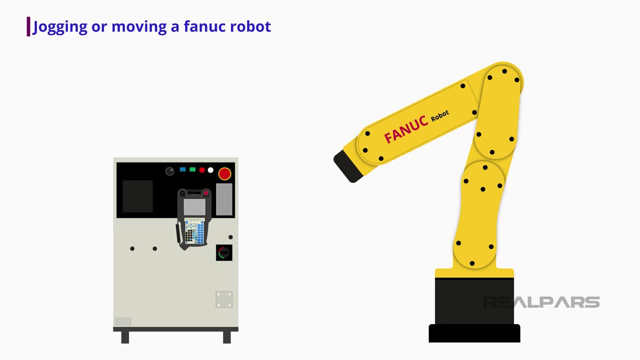 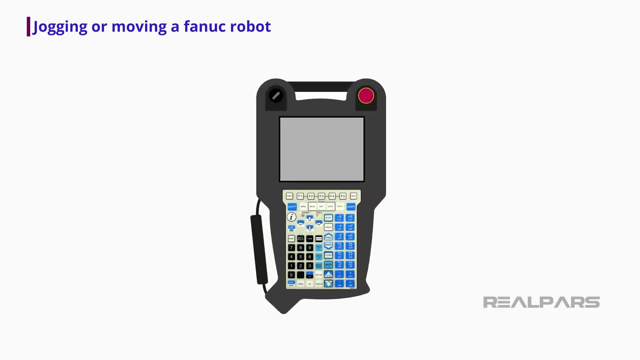 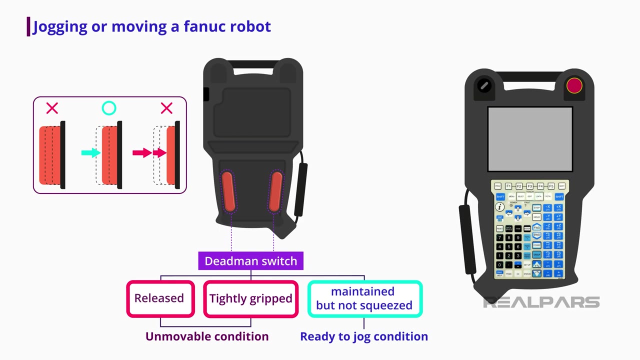 I will now describe how to jog a robot that has been shipped from the factory without any setup or configuration. To jog the robot, you will need to understand how the deadman switch works. The deadman switch is a three position switch. When in the released or tightly gripped position. 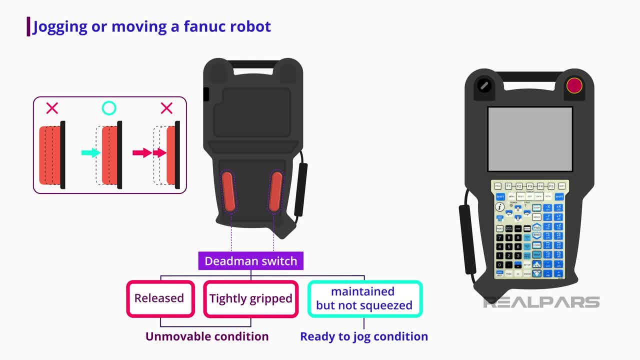 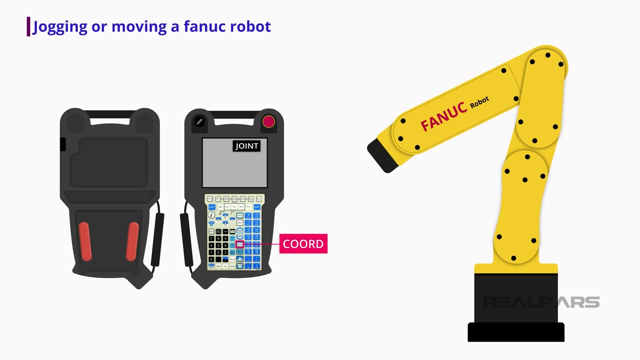 the robot is in an unmovable condition. When the deadman switch is maintained but not squeezed, the robot's servos will release, which enables jogging To jog. press the coordinate key until the display on the top right black square reads JOINT. 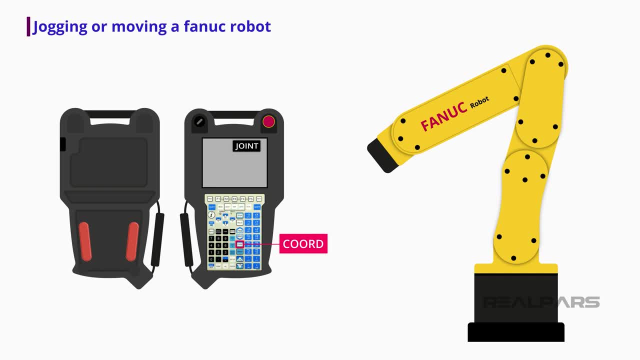 This tells the robot to only move one joint at a time. While the deadman switch is being pressed and one of the shift keys is also being pressed, you can press a J1 minus or J1 plus key to move the robot on J1.. 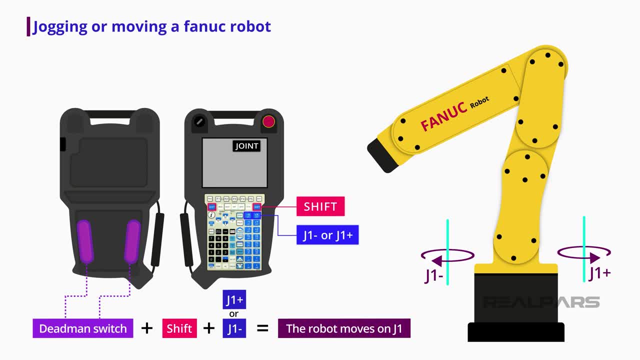 It is important to note that each time the robot is jogged or moved, the deadman and shift key must be maintained, because if either the shift key or deadman switch is pressed, the deadman switch is released, then the process must be repeated.